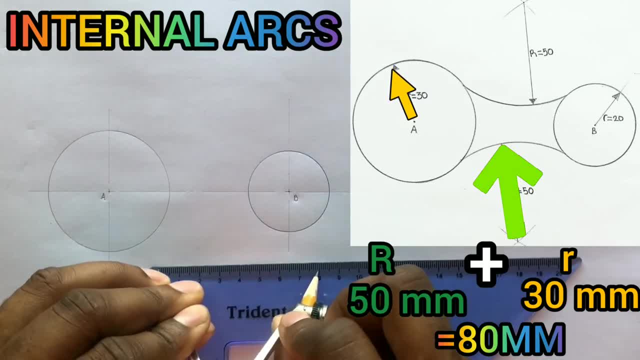 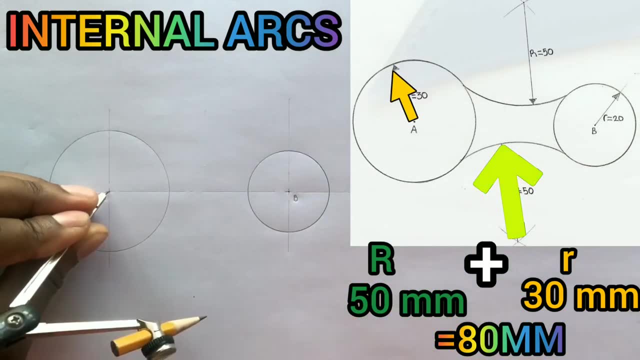 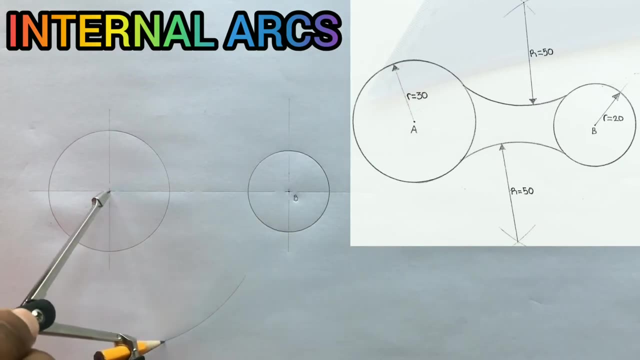 Now open your compass to 80mm and, using A as the center, scribe an arc below the two circles. Again, you need to add radius 50 plus radius 30.. Now open your compass to a radius of 80mm and, from the center B, scribe another circle. 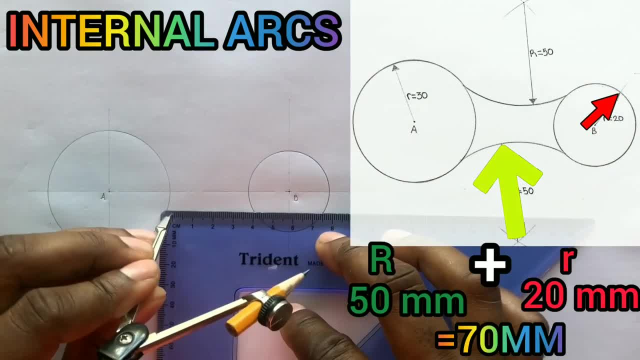 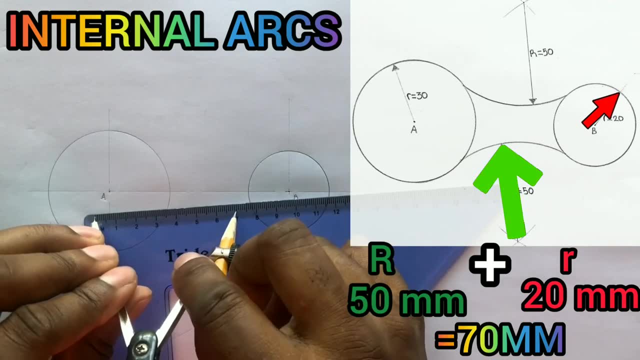 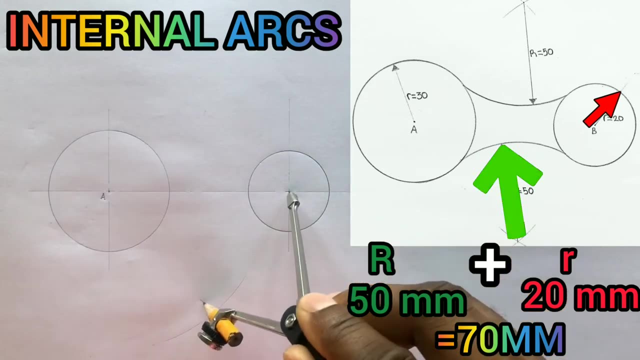 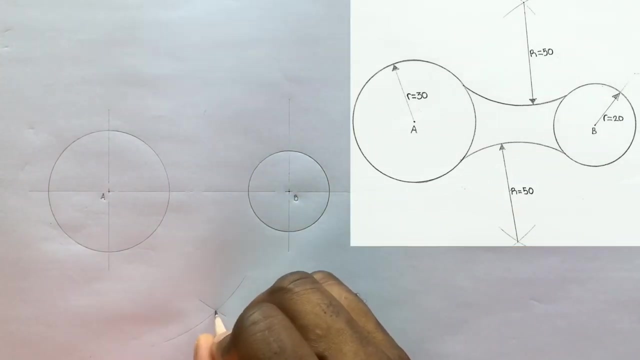 Again, you need to add radius 50 plus radius 20 to give you 70mm. Now open your compass to a radius of 70mm and from B, you will scribe an arc. This intersection is very important. Identify this intersection and label it: O. Now, from this intersection, you will scribe: 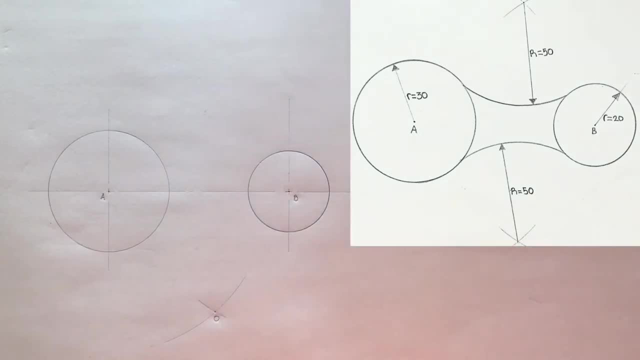 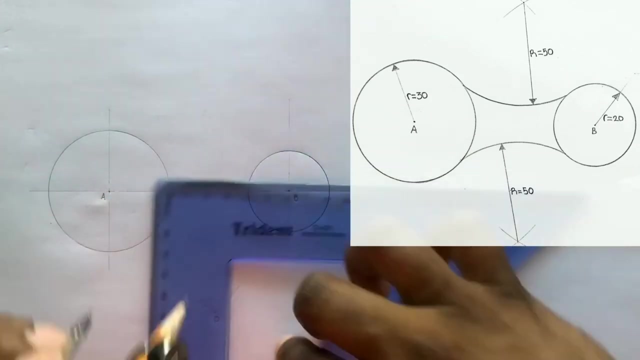 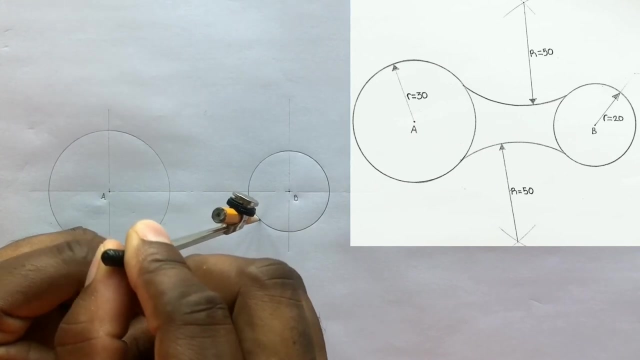 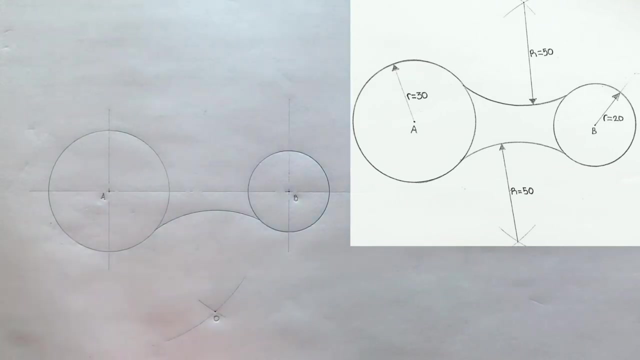 internal arc of radius 50. Open your compass to a radius of 50 and draw your internal arc to blend these two circles. You have just drawn your internal arc, which falls on the inside of these two circles, blending them together nice and neat. Now repeat this procedure at the. 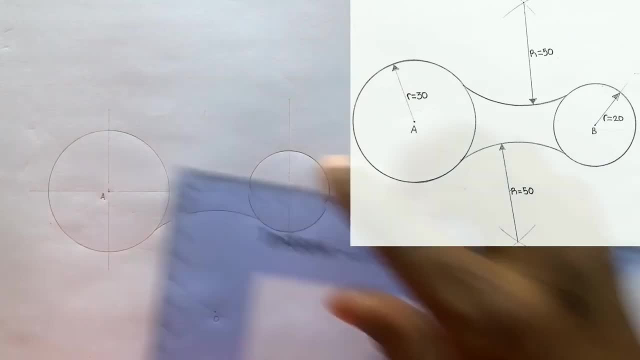 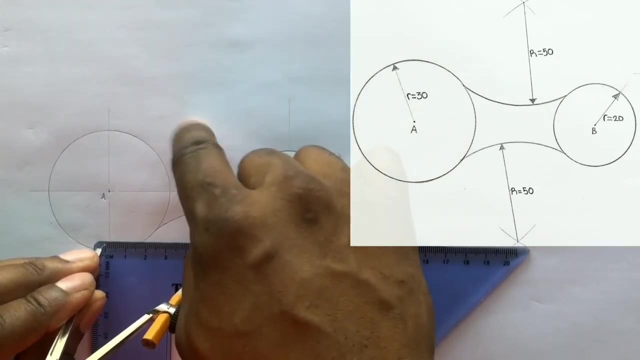 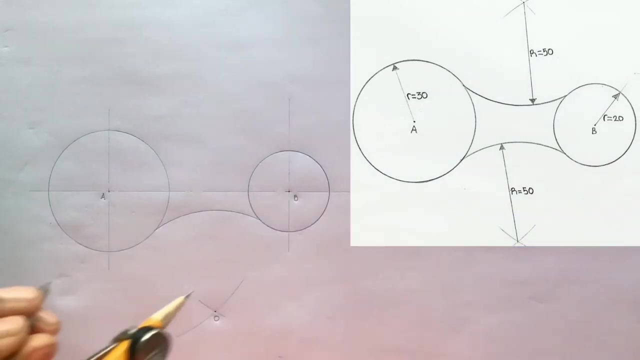 top for additional practice. So what you will do is to open your compass to a radius of 80 millimeters, which is the addition of radius 50 and radius 30. And from the center, A scribe, an arc above the two circles, Once more open. 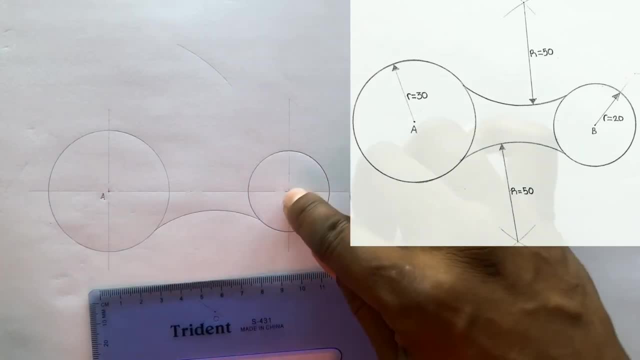 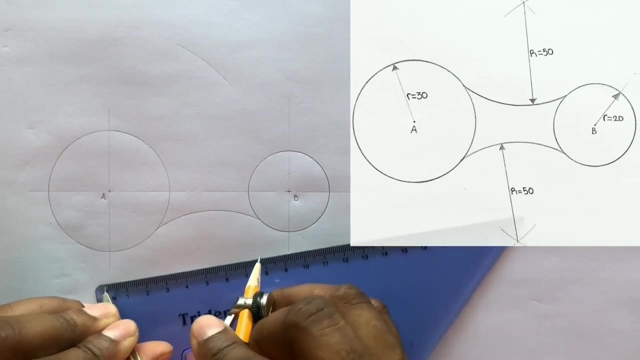 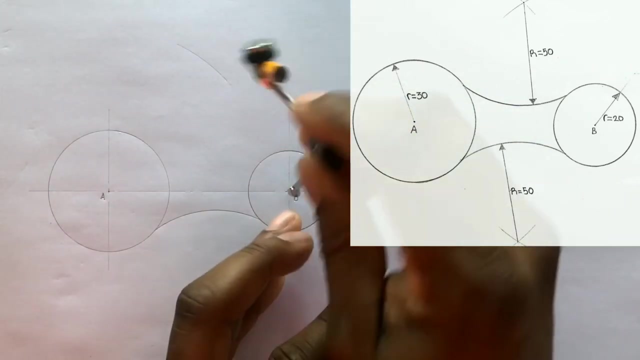 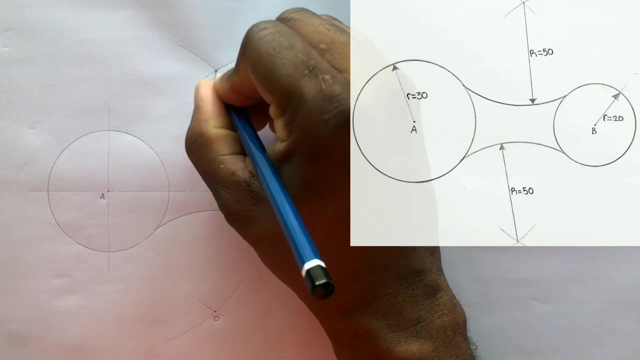 your compass to the sum of radius 20 millimeters plus radius 50 millimeters, giving you a total of 70 millimeters. And from the center B, scribe an arc above to intersect the previous arc. you drew Great. Now identify the center and label it as O. Now both internal arcs are.